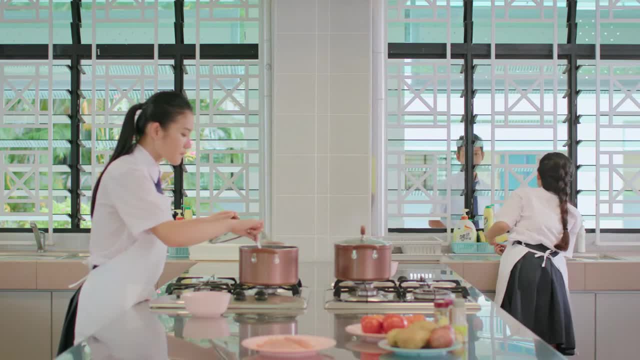 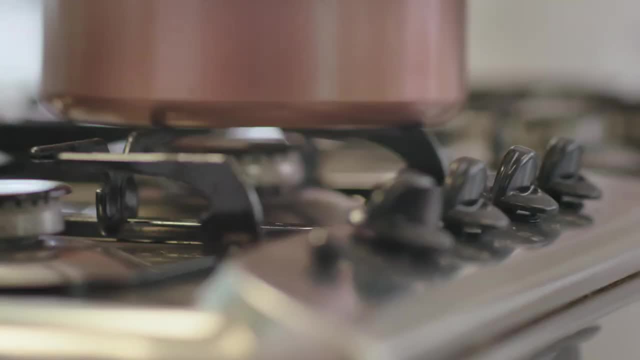 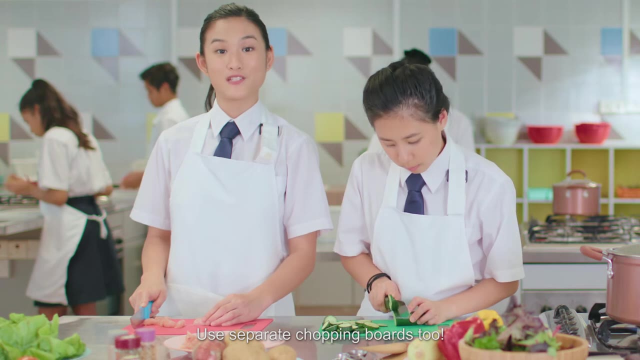 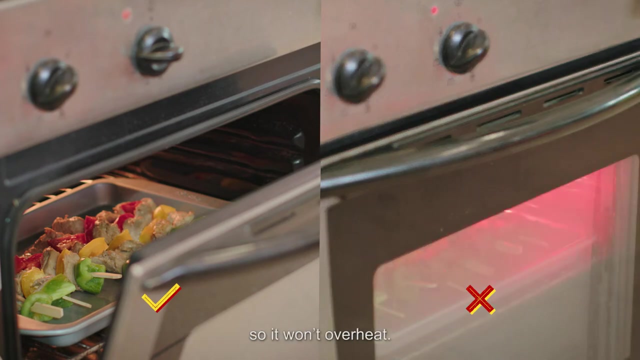 Wash the stove when cooking And turn it off before you go. Keep raw food and ready-to-eat food apart. Use separate chopping boards too. Leave the oven door ajar during grilling so it won't overheat. Before frying, dry all cooking utensils. 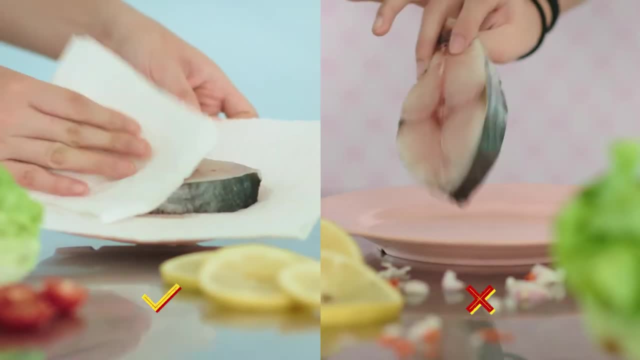 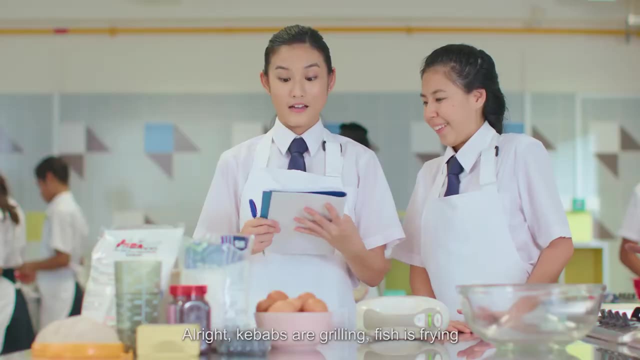 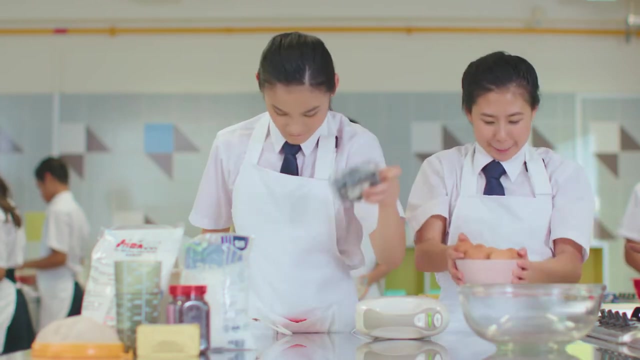 and the food for frying. When frying, slide food gently into hot oil. Alright, kebabs are grilling, fish is frying. And now for the last dish, dessert. If an electrical appliance is faulty, inform the teacher and do not use it. 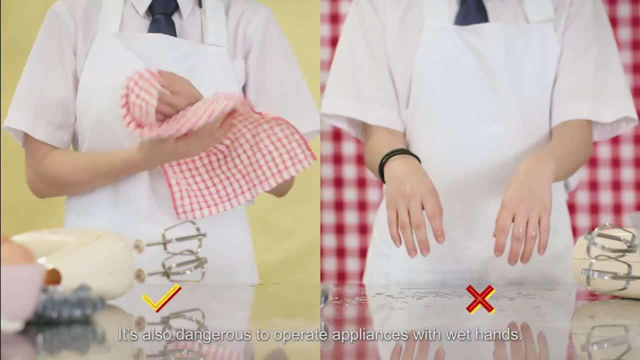 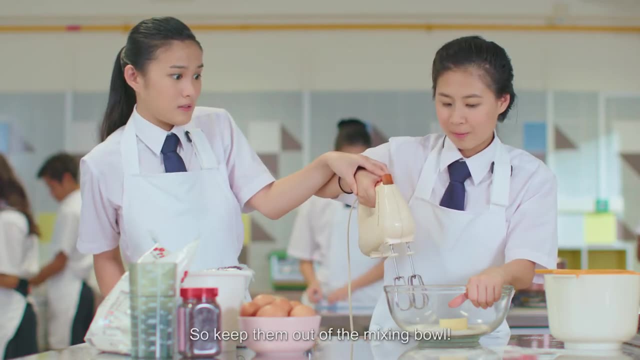 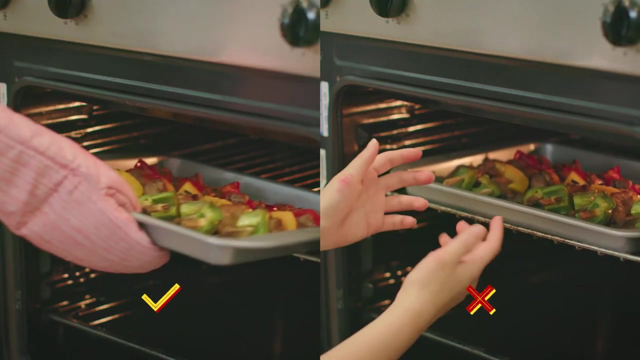 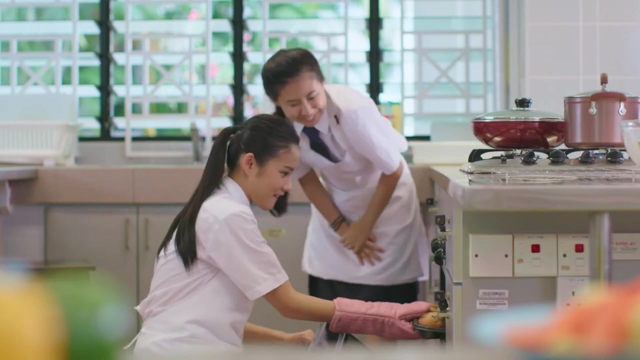 It's dangerous. It's also dangerous to operate appliances with wet hands. Your hands are precious, So keep them out of the mixing bowl And wear oven gloves when you take food out of the oven. The muffins are late. Make sure they are thoroughly cooked. 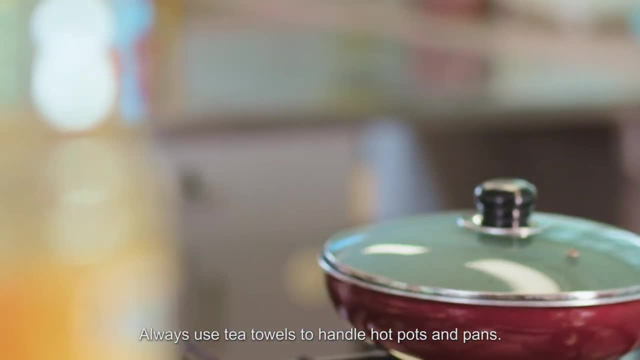 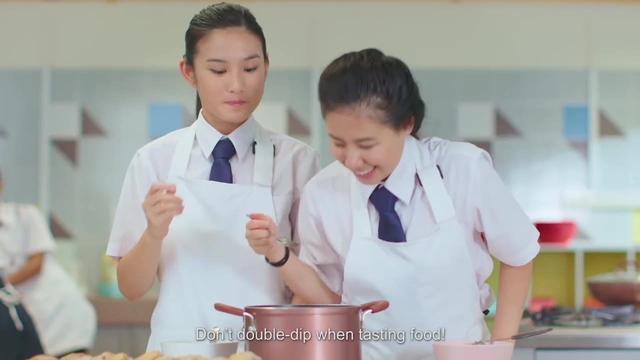 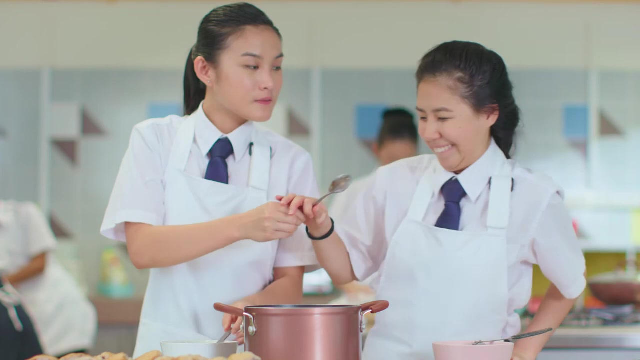 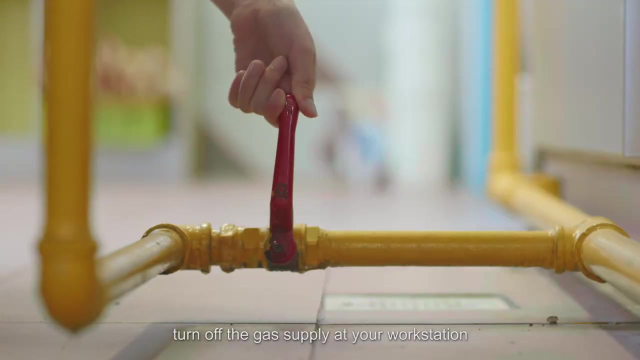 Always use tea towels to handle hot pots and pans. Don't double dip when tasting food, Even if it tastes so good. If you spill something, clean it up immediately. Finally, turn off the gas supply at your workstation and clear the trash. 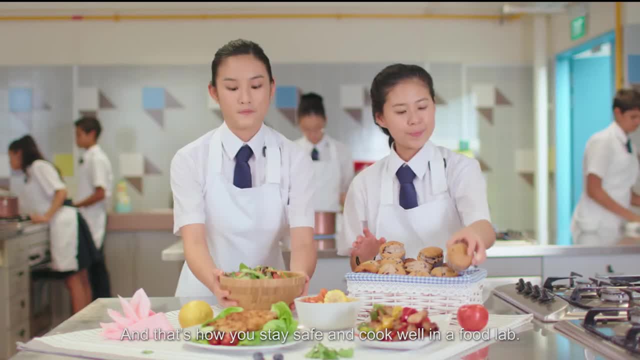 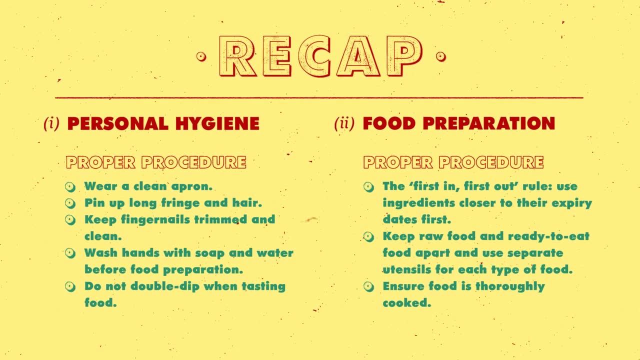 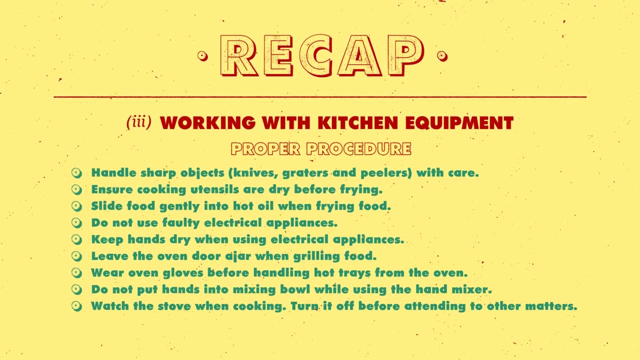 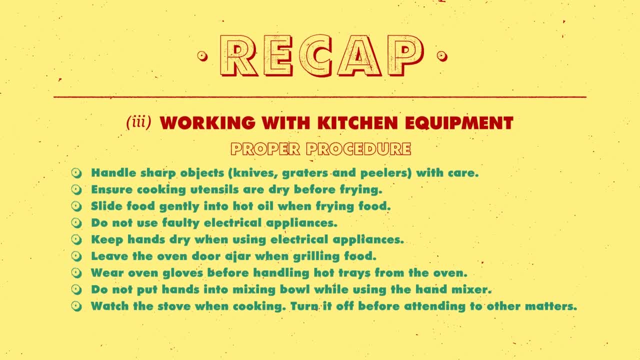 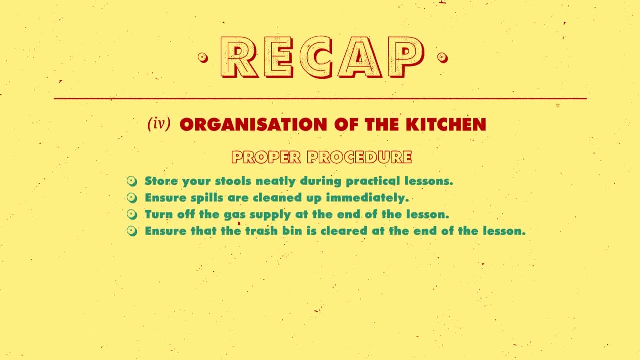 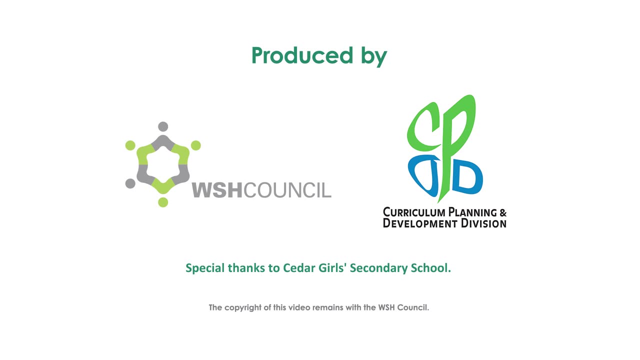